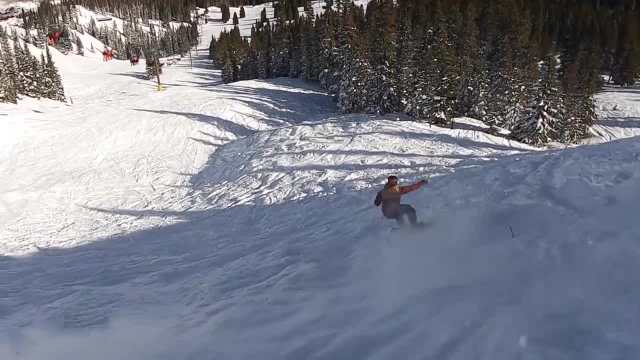 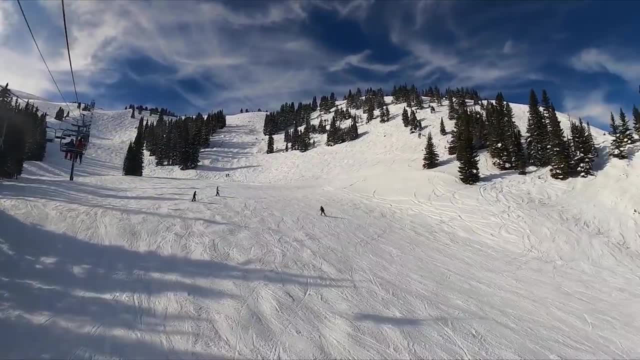 slope. So today we're going to talk about exactly how to ride steeper terrain. Now the first thing you have to think about is run selection. So you can see, the bottom of this run is grooved but the top is not, So it's kind of powdery snow and bogles. This isn't the first. 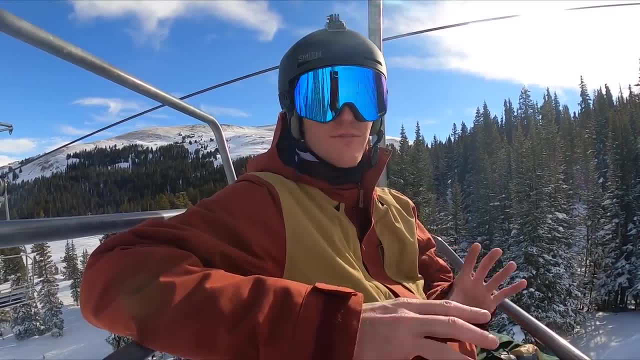 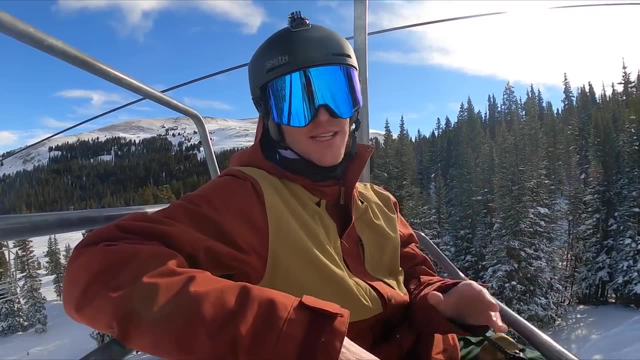 kind of black diamond or double black diamond. you want to go down. You can find a steep run that's perfectly groomed and corduroy and start there. Now I know some smaller mountains, maybe the black diamonds. they leave them ungroomed and you have. 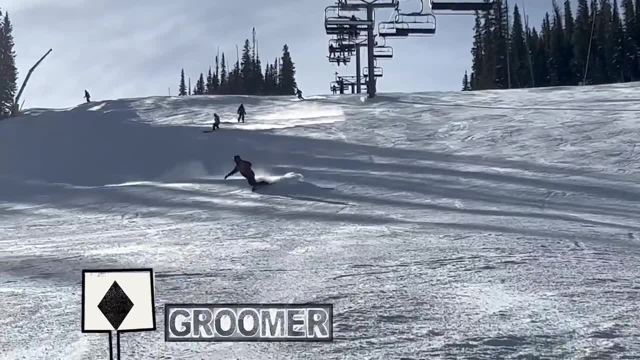 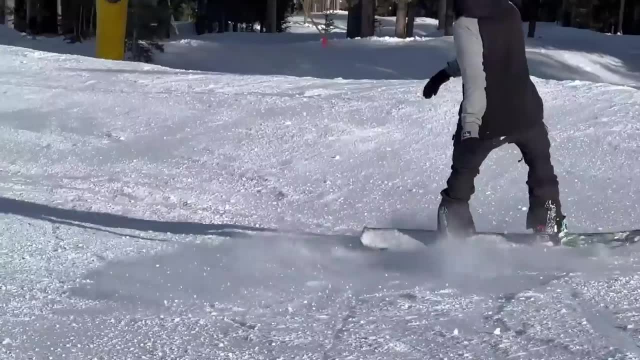 no choice But, if possible, find a groomer. that's a black diamond, And we're first just going to play with that increased speed before we have to deal with variable conditions. So the first thing you need to understand: if your edge points down the hill, you're going to gain more speed and it's 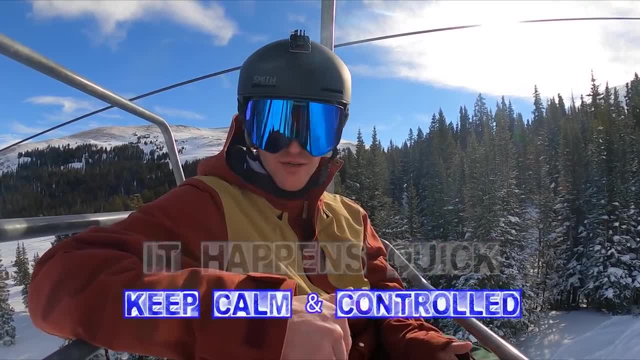 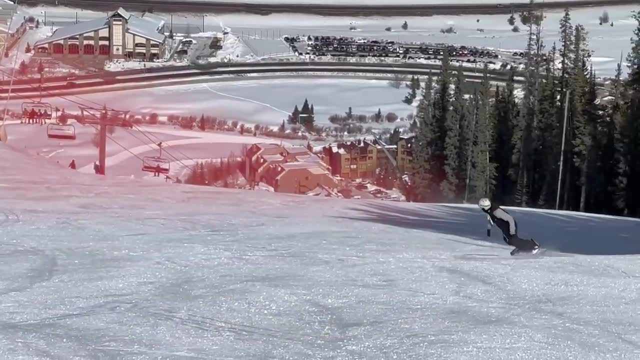 going to happen much more rapidly than on a blue square or a green circle. So what we want to do is get your edge pointed across the slope. Now you might look at the trees on the left side or the right side of the slope and just point your edge right there, As long as your edge is sideways on. 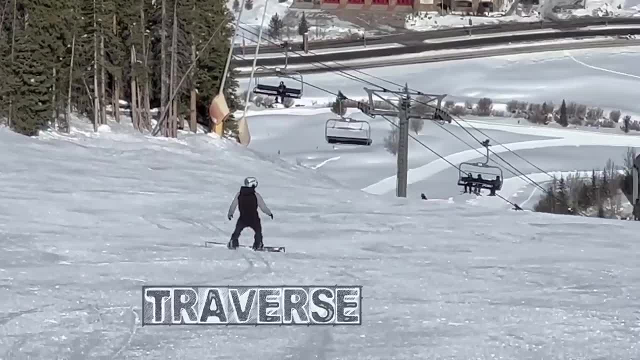 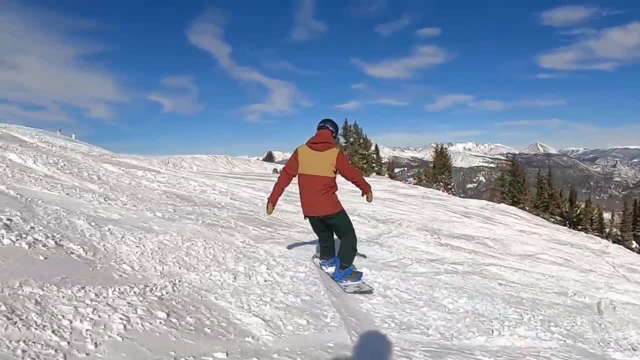 the slope, you're not going to go anywhere. You can do what's called a traverse, which is where you're carrying your momentum across the slope rather than down the hill. Now, when you want to get up more speed, you're going to point the edge further down the fall line than you had it when. 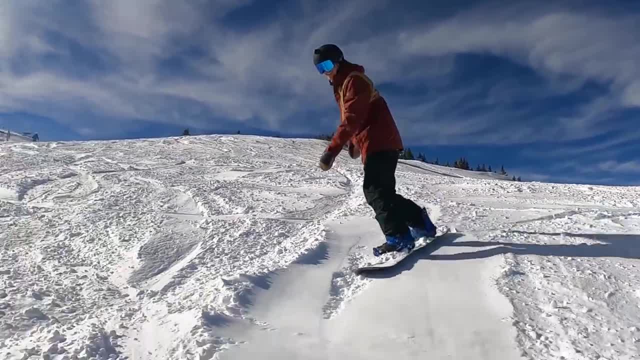 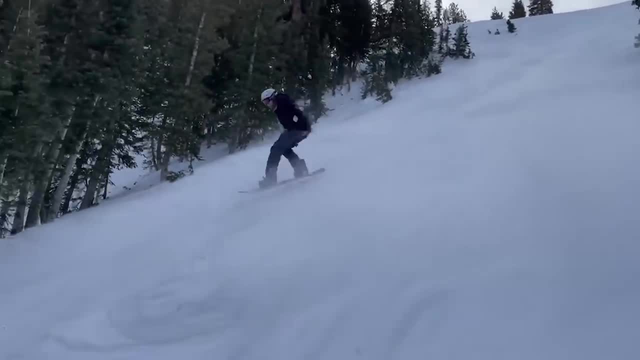 you're traversing And again you're going to pick up speed really rapidly. So if this starts to be completely sideways, again, that's going to stop. So anytime you need to stop, just counter rotate, turn your board completely sideways on the run and then take that momentum If you're still. 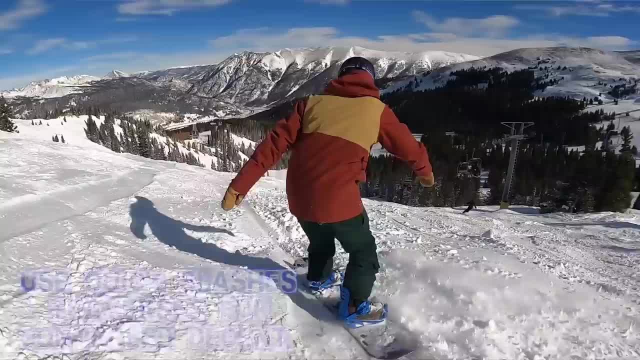 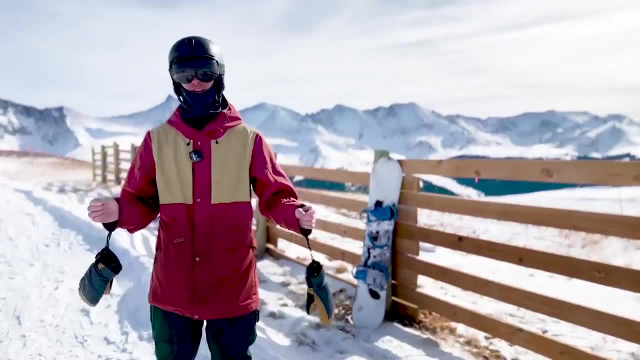 sliding down the hill and you put it into a traverse so that that extra energy gets carried across the slope rather than you just skidding straight down, even though you're turned sideways. that's going to help a lot. What up, Shredder. We interrupt this for a brief commercial announcement. 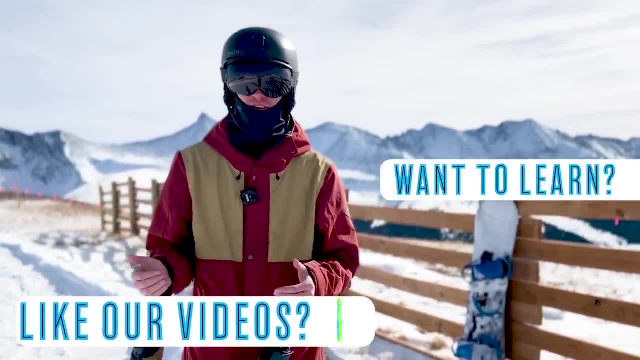 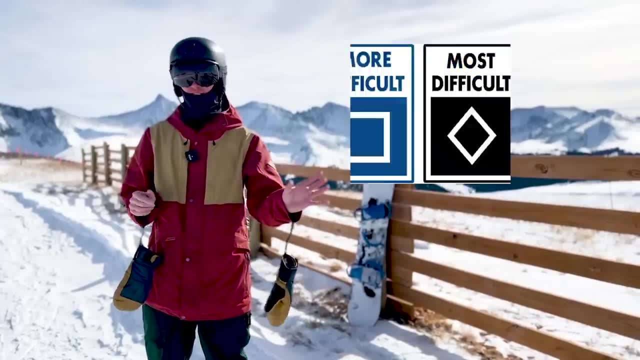 If you like what you're watching right now and you are a complete beginner at snowboarding and you want success to get better, so you can go out there and make turns on the whole mountain, from green circles to double black diamonds, we've got a 28-piece series to take you from learning how to. 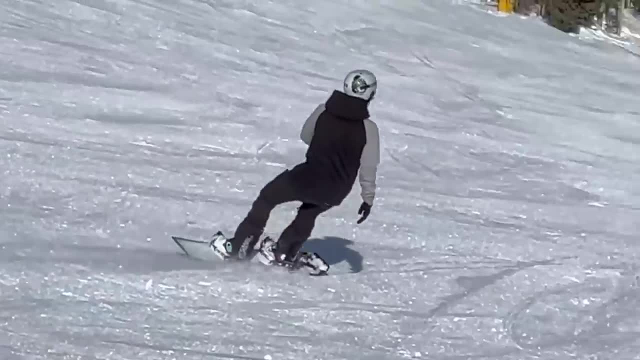 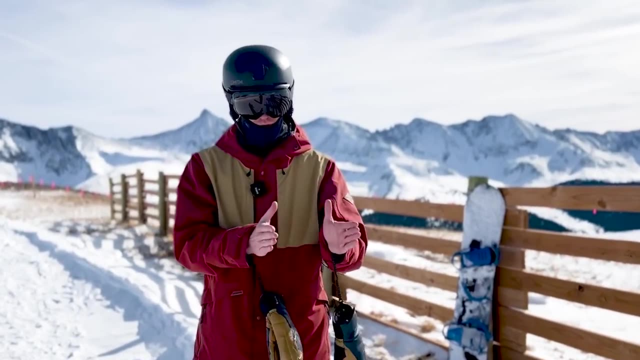 get on the list to link those turns to start to do your first butters inside of Shred School. So the best way to support us, if you like our channel, is to go sign up for Shred School right now. You're going to get that beginner series and you can start working through step by step. All right. 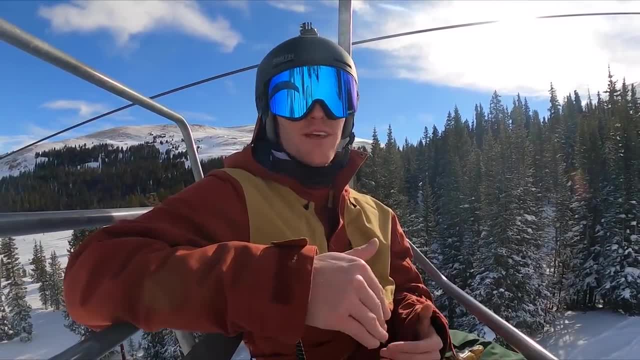 back to your video. Okay, so now we want to get up some speed. Now some people think that you can't carve without picking up a ton of speed, and that's just not the case. But if you're a beginner and you 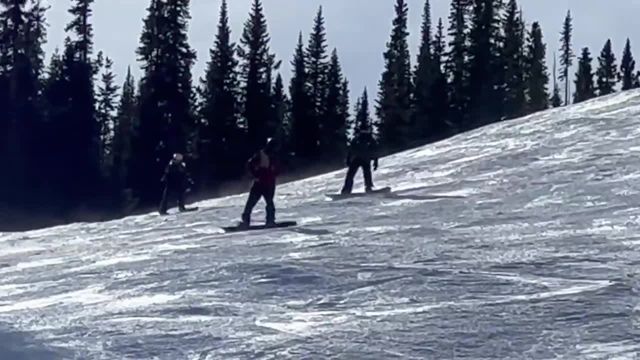 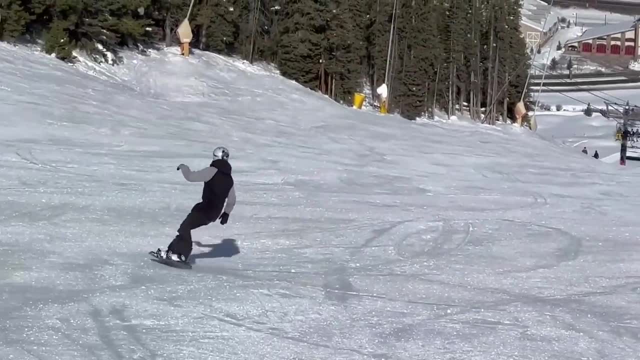 don't know how to do that. that's not true. We just want our carves to look more like traverses. So instead of pointing your edge down the hill when we start to carve, we're going to do a traverse on our toe side edge and then we're going to do a quick turn to our heels. A quick carve we can. 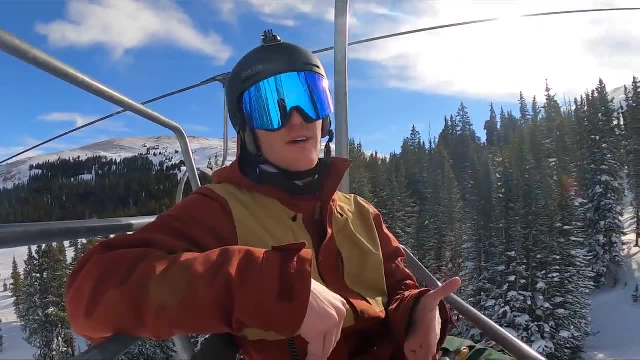 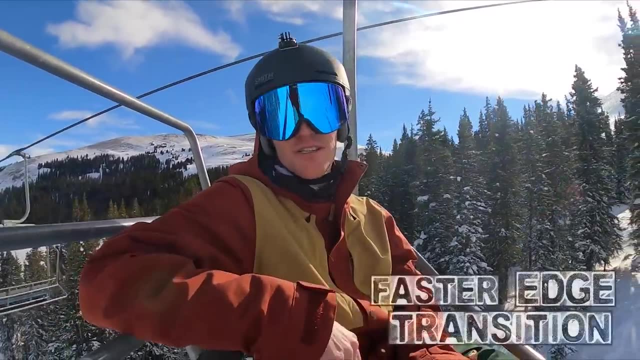 stay on our edge and then we're going to heel side traverse. Now we're still going to be carving because we're using the side cut of our snowboard. We're carrying our energy across the hill. So the key here is you have to make those edge transitions faster than you would on a mellow or slope. The 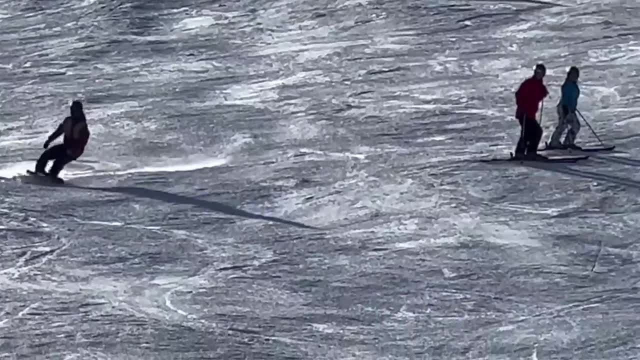 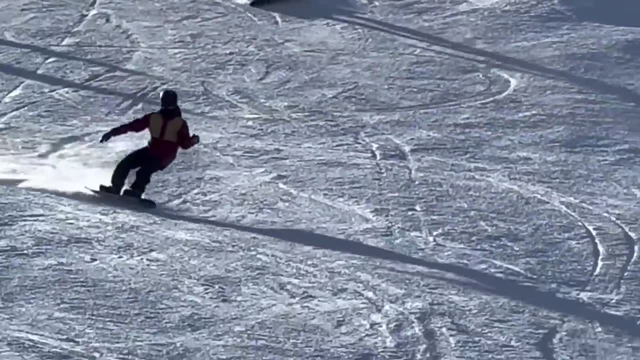 faster you can make that transition, the less you have to worry about the momentum getting right down the hill. So when we get confident, we're going to start to point our carves a little bit more down the hill. Now this is going to feel really good, especially under groomer, You can. 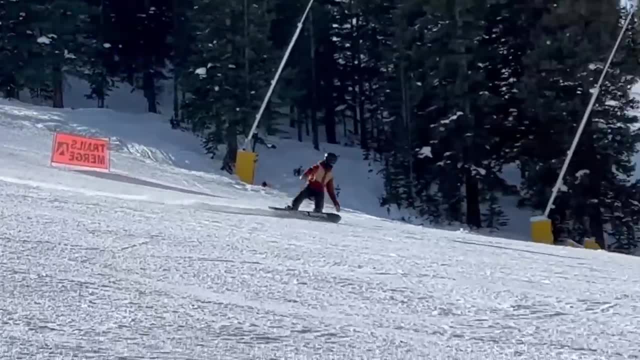 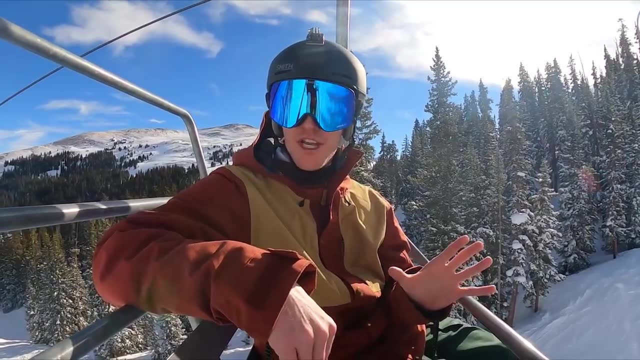 start to get some speed up, but when you get too much speed we're going to throw in counter rotation. So try to do carves on your edge, where the edge is carrying you across the slope, and then, when you get too much speed, throw in counter rotation in between your carves. You don't have to. 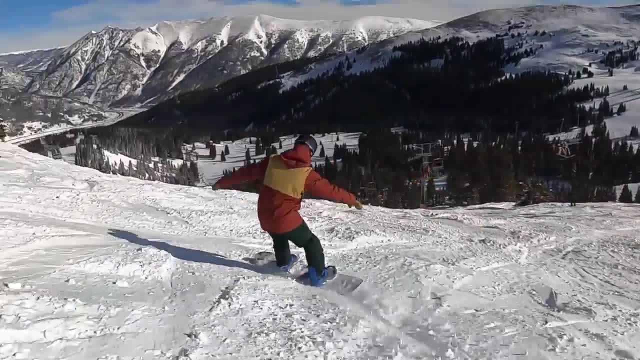 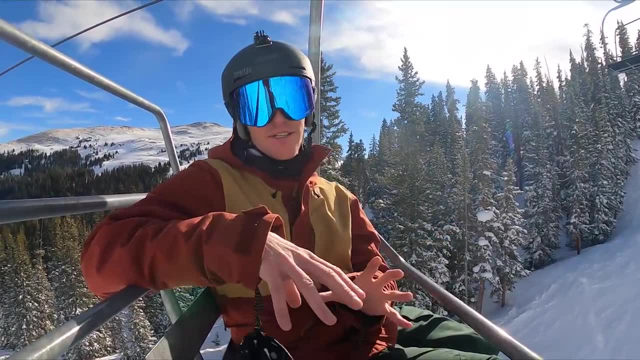 stop carving completely but just slash it out. Turn that forward sideways. that's going to cut speed. If you have way too much speed, turn it completely sideways and traverse across the slope. Remember, if you just turn sideways to cut your speed but you don't traverse, the momentum is. 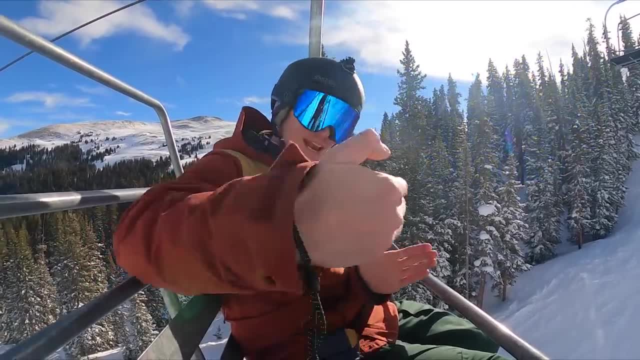 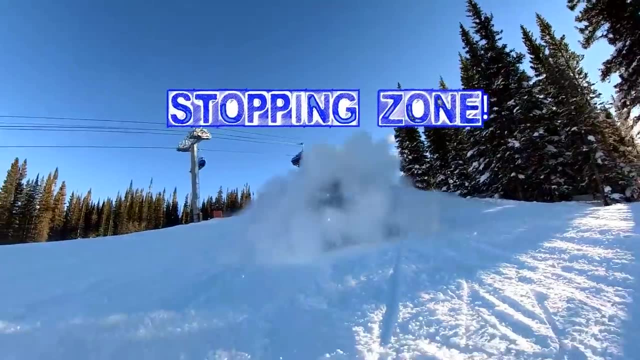 still going to carry you down the hill. So when you turn sideways, go into a traverse and let it carry itself out towards the trees on the side of the run. The next thing we got to worry about is our stopping zone. So especially when the terrain becomes variable, that means moguls powder. 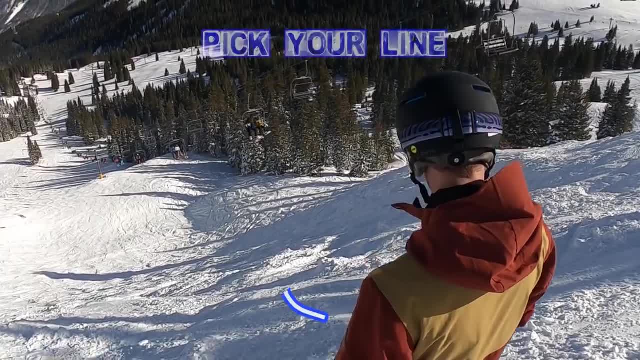 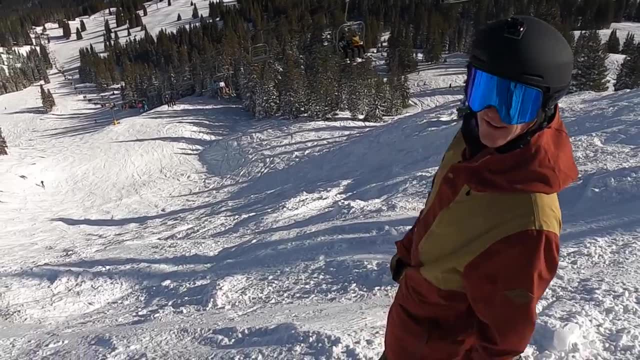 things like that. When we start going faster, we might have to see our line out. That means we're taking a line where we can't stop at any point in the line. We have to wait until it's over. Maybe we have an area we don't want to be in, And so what I like to do is I up my stopping zone first. 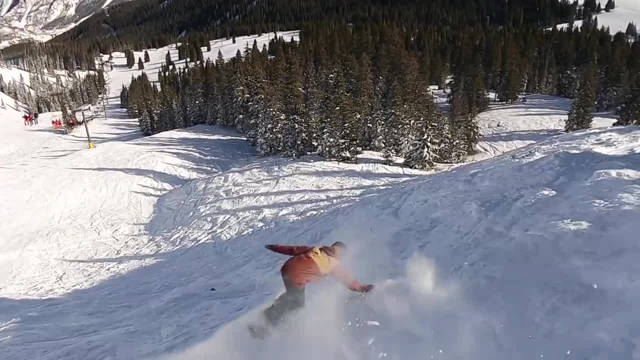 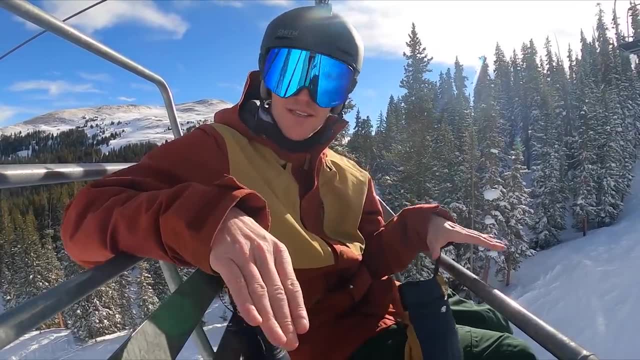 from my starting point and then I'm going to say, okay, I'm going to stop down there until I get to that point. I'm going to carry my speed fast, And so I can have a really fast line, knowing that there's a clear space to stop. Now, a good stopping zone is an area that doesn't have trees in it. 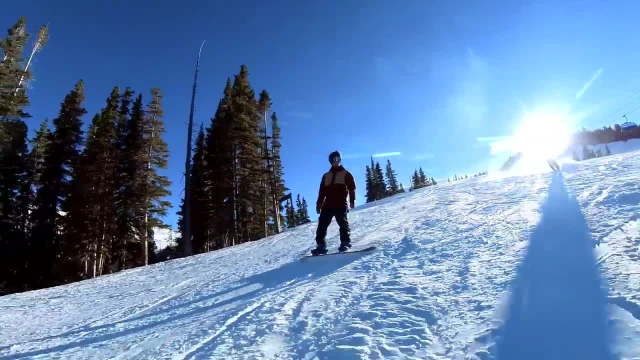 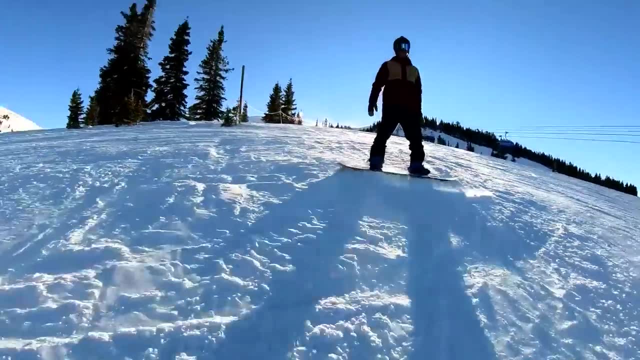 that doesn't have bumps and it's just a smooth, preferably flat, but it could be steep area- but just a smooth area where you can actually turn sideways and your snowboard can carry out that momentum without you hitting a bump. So that's what I like to do. I like to do that. 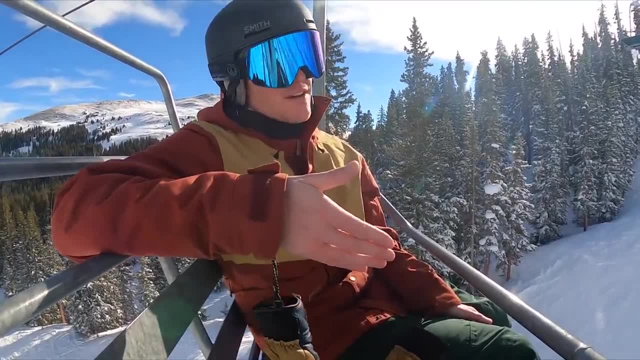 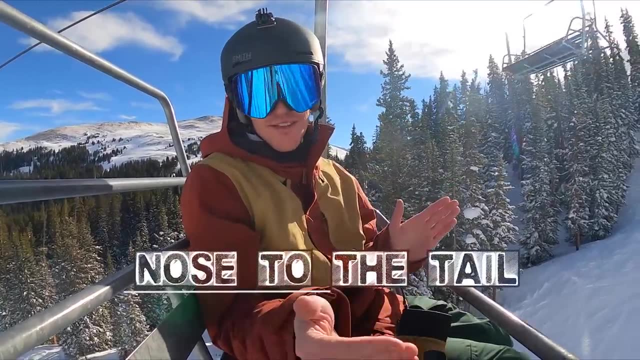 Without you hitting big bumps and it just bumping you up. One thing I want to mention here is when you are riding bumps down a black diamond or double black diamond, you want the energy to disperse through your board from the nose to the tail, not from the toe side edge to the heel side. 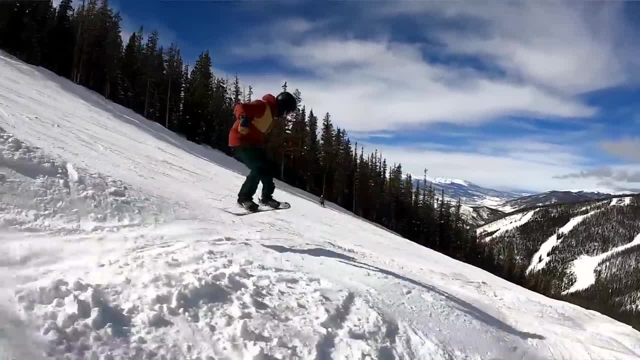 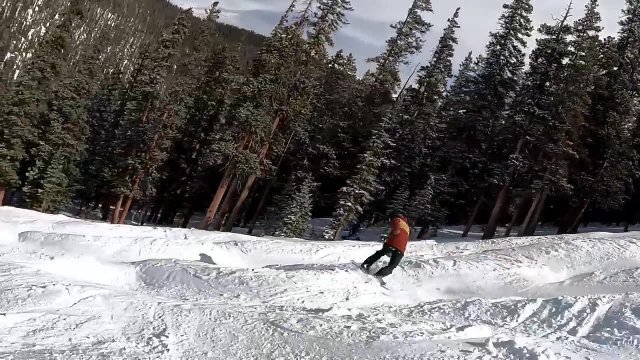 edge or the heel side edge to the toe side edge. The most stable position is to use your whole snowboard to disperse those bumps, And so that means pointing the board forward over those bumps rather than sideways. You see, a lot of people just like going over bumps sideways and getting bucked. 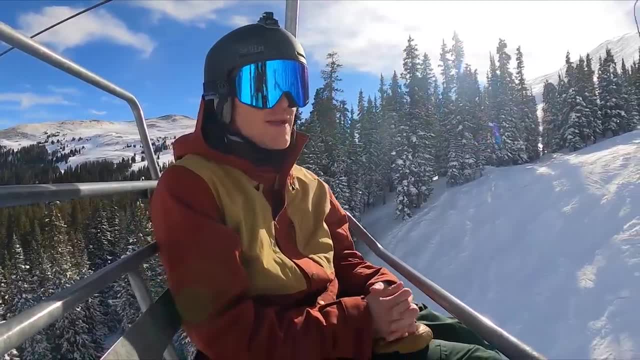 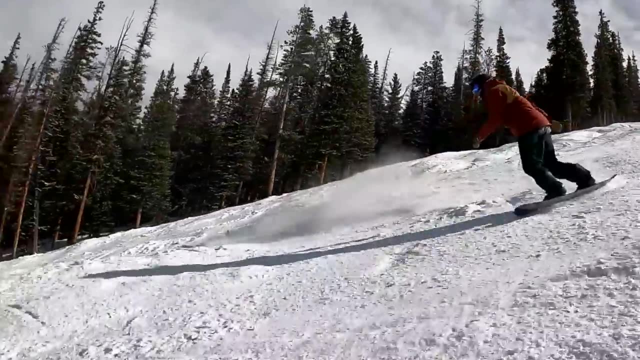 and then they fall on their butt or their stomach or whatever. So the easiest way to avoid that is: take the, take the bump with your board going forward And then, after you get over the bump, then turn sideways to cut the speed. So up here I can see the whole line below me and I'm going to scope out what is like feasible for. 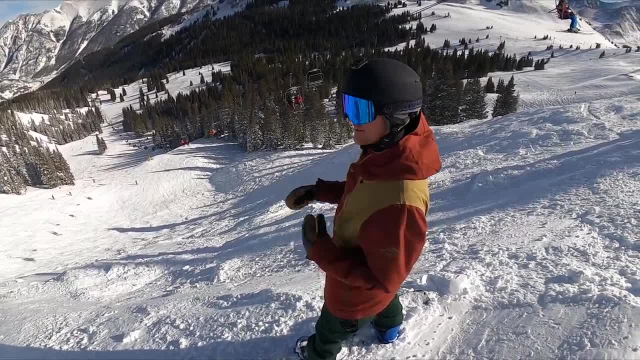 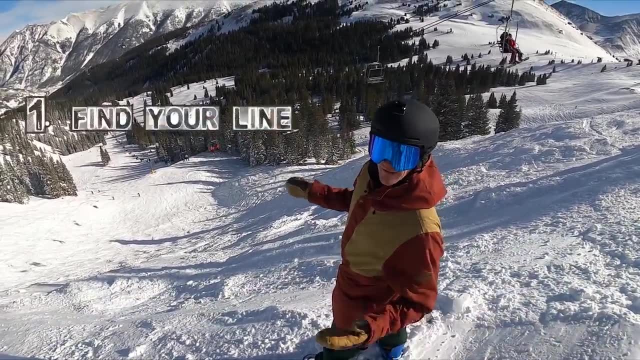 me to go down with my ability level. So I'm going to look for a line that's easy enough for me to handle, Not too difficult, because there usually are choices on runs like this. Once I find my line, I'm going to find my stopping zone. You can see that flat area down below. I'm going to expect. 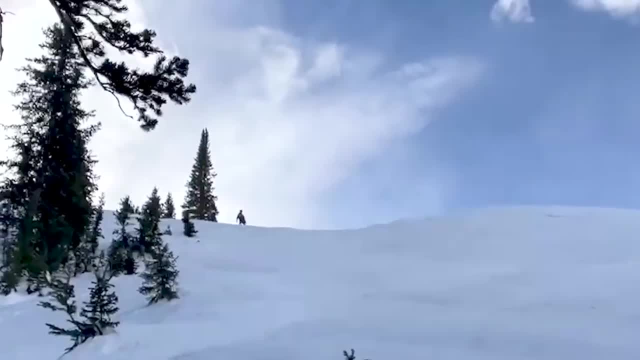 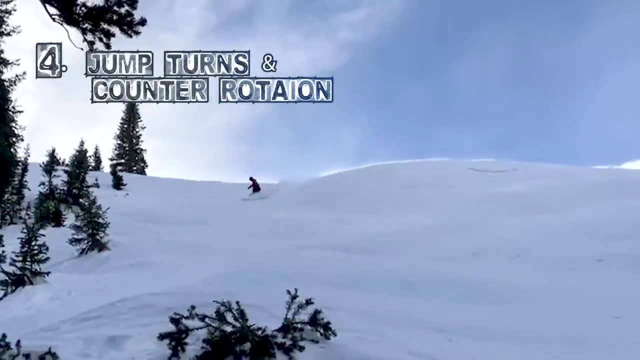 to charge this until I get there. Now it is really steep, So to control my speed I'm going to keep my board as sideways as possible on the run. I'm going to use maybe even some jump turns and a lot of counter rotation on this because I'm not going to be doing carves because it's so bumpy. So mainly, 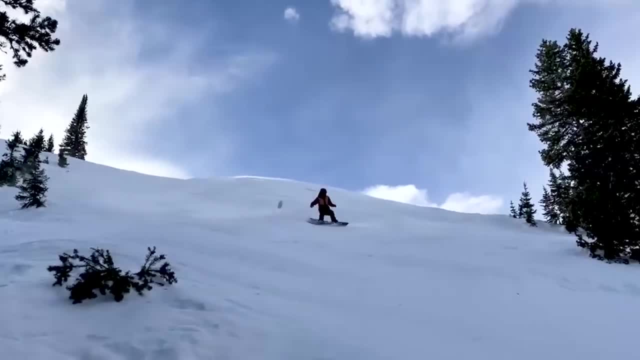 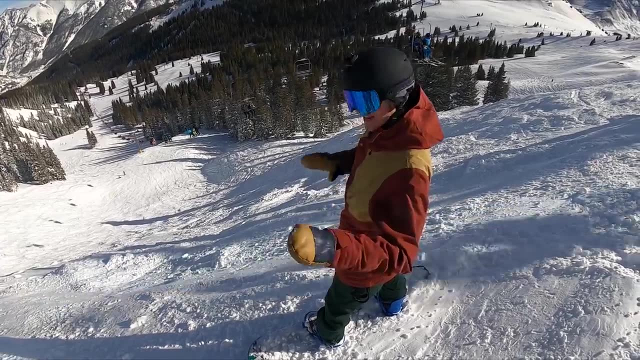 going to be traversing and jump turns and counter rotation, keeping my board sideways. When I see a clear line to the stopping zone, I might point it out straight, catch up a lot more speed and then go into that controlled stop. Go out there, give these a shot. Let us know in the comments. does this help? That's all for today. Peace out Shredder.